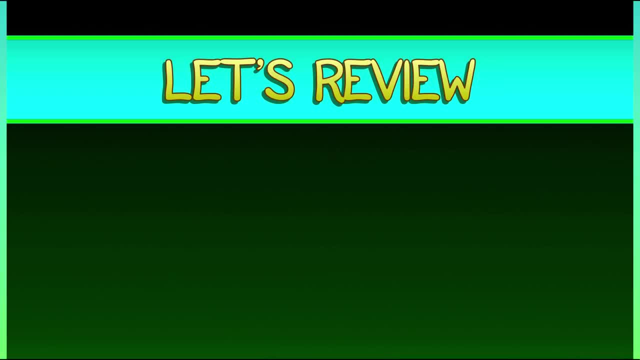 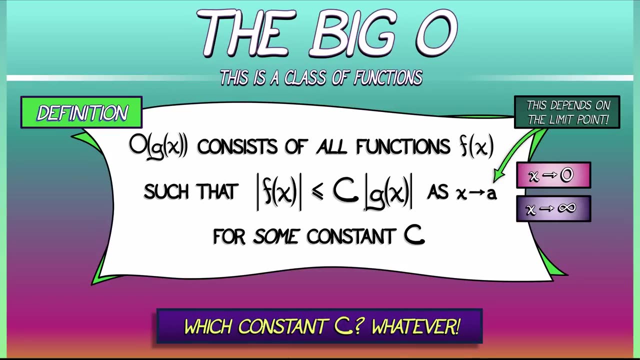 Let's review what big O means and how it works in some simple cases. For starters, let's go back to the definition. Big O is a class of functions. Big O of g of x consists of all functions f of x, such that f is bounded by g times some constant c, everything in absolute. 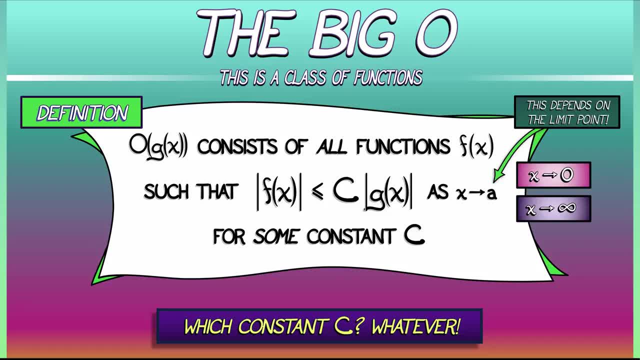 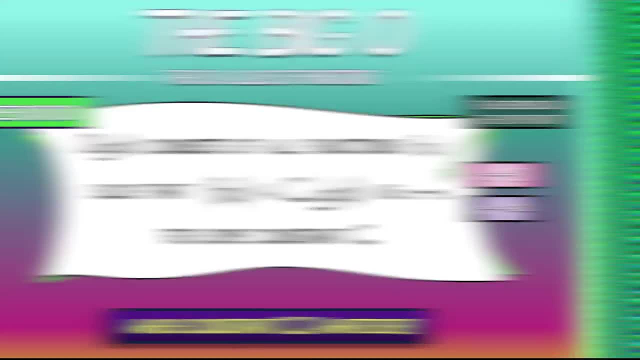 value in the limit. Maybe it's going to zero, Maybe it's going to infinity. Oh, it's kind of a mouthful. Things you got to remember. Don't forget the absolute values, Don't forget about the constant c. but it doesn't matter what the constant c is. That's the definition. But what? 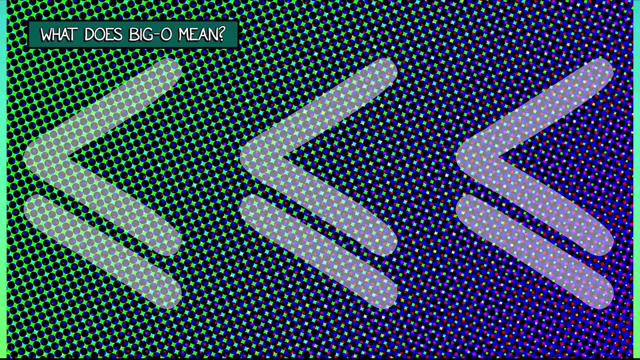 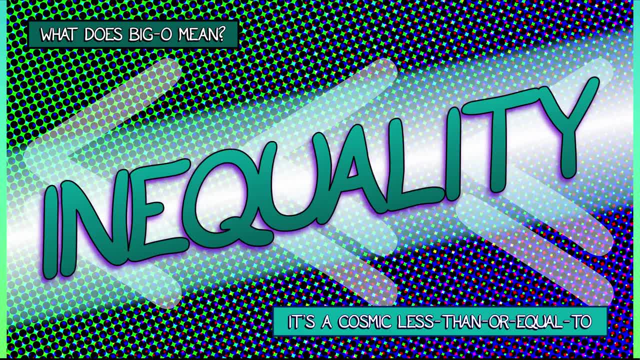 does it mean Big O can be very profitably thought of in terms of that inequality. It's kind of like a cosmic less than or equal to sign, And indeed when you're trying to figure out what belongs in big O of something else, 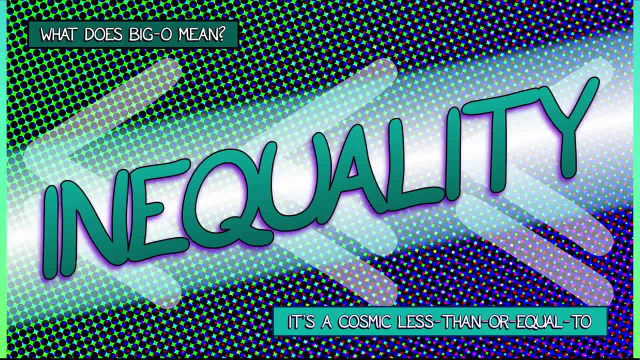 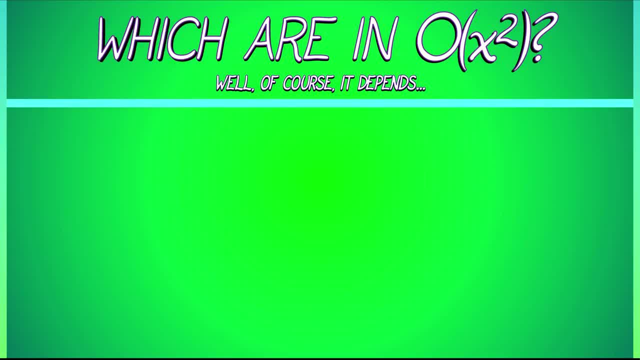 you're going to be thinking in terms of inequalities. So, for example, which of the following functions are, in big O of x squared? Well, of course it depends. It depends on, let's say, whether we're talking about the limit where x is going to zero, or 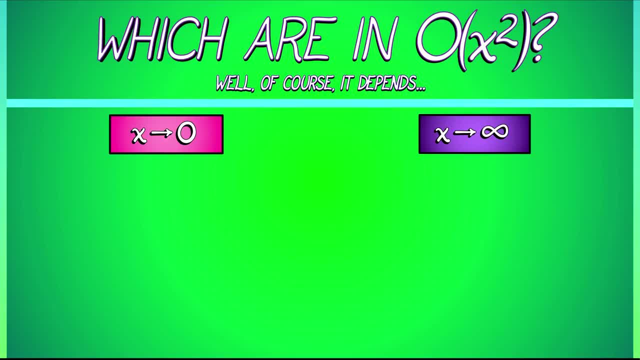 the limit where x is going to infinity. So, for example, if we consider the function x cubed and say: is that in big O of x squared Well in the limit as x goes to zero? what we need to answer is whether or not there's some constant c so that x cubed is less than or equal to c times x. 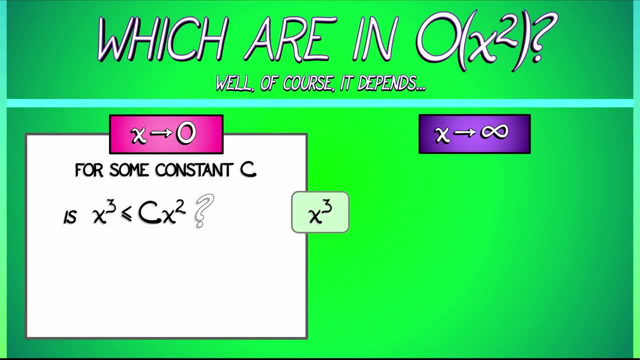 squared And let's assume that x is a small positive number here, so that we don't have to write a whole bunch of absolute value signs. Well, does that work? If x is a really tiny positive number, then x cubed is tiny, And if x is a small positive number, then x cubed is a small positive. 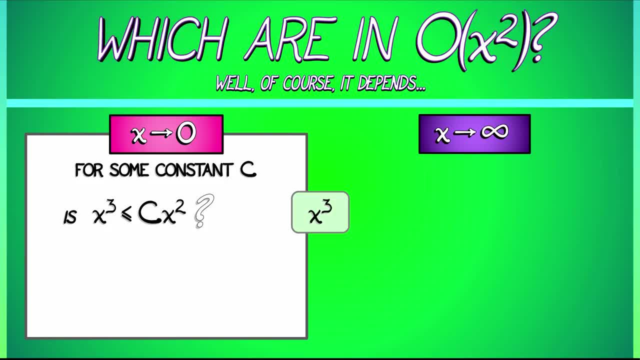 times tiny, times tiny, and that's much smaller than x squared, no matter what constant you pick in the limit, as x goes to 0, the quadratic bounds, the cubic. so x cubed is in big O of x squared as x goes to 0. but as x goes to infinity is there. 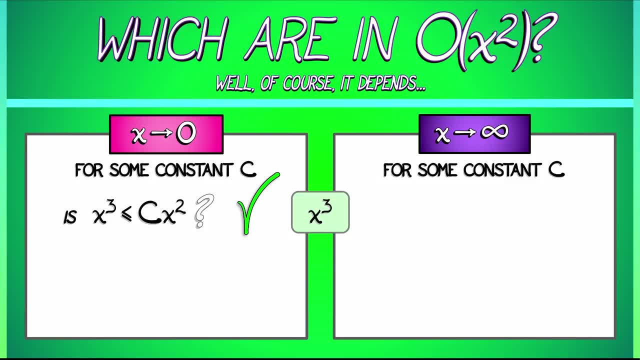 some constant C so that x cubed is bounded above by that. constant times x squared- no, uh-uh, not happening. if x is some really really large number, then x times x times x is definitely going to dominate. x squared times a constant, no matter what constant C you pick. it could be really huge, but eventually x is going. 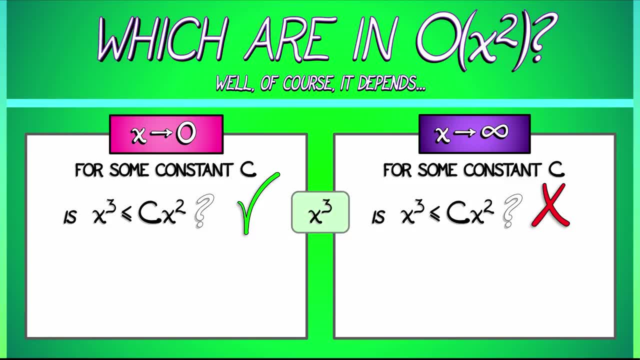 to get large enough to dominate it. so x cubed, not in big O of x squared as x goes to infinity. now at this point you might be thinking, oh, I get it for any function in the limit as x goes to infinity, but it's not going to be. 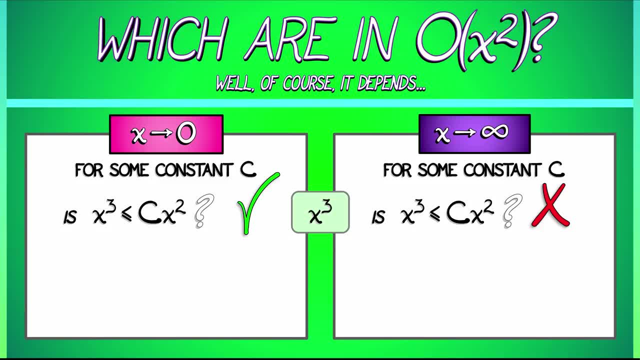 in big O of x squared in one limit, but not the other. well, let's think. consider the function e to the x. is that in big O of x squared well, as x goes to infinity? absolutely not. we know that the exponential functions absolutely dominate all polynomial functions. there's no way that e to the x is less. 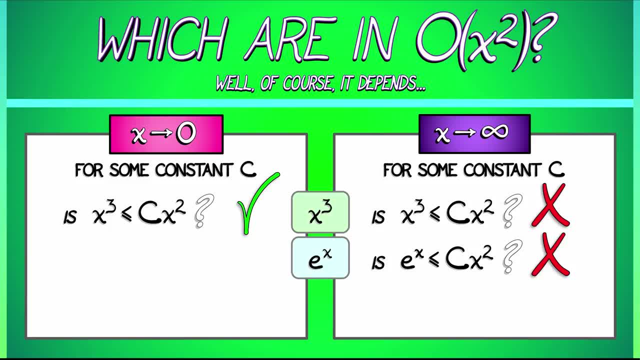 than any constant times. x squared, so e to the x, not in big O of x squared as x goes to infinity. however, what happens in the limit as x goes to zero? ah, let me think. um x squared is going to zero, but e to the x is is going to 1, there's no way. 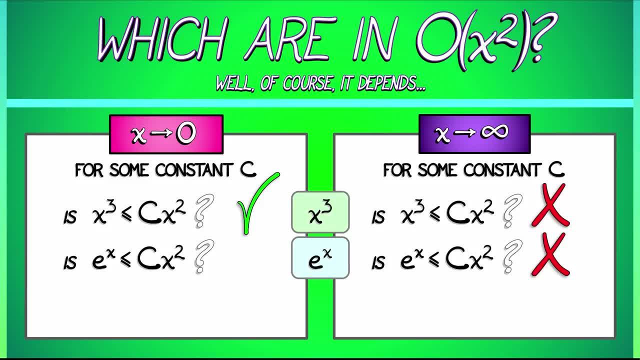 that there's some constant, so that e to the x is less than that constant times x squared in the limit as x goes to 0. so this function, e to the x, is not in big O of x squared as x goes to 0 or is a constant times x squared as x does zero. 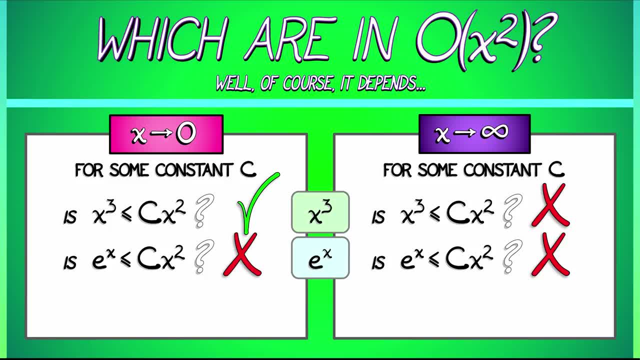 as x goes to infinity. Now I'll leave it to you to try to figure out. is there a function that is in big O of x, squared in both limits, as x goes to zero and as x goes to infinity? I don't know. 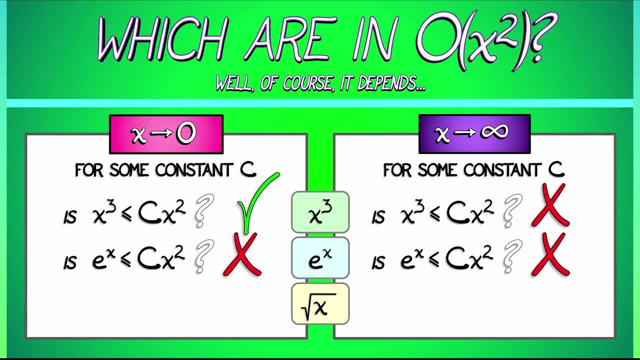 What about square root of x? Let's see, Is square root of x dominated by x squared in the limit as x goes to zero? No, no, that square root of x. it does go to zero in the limit, but it remains.